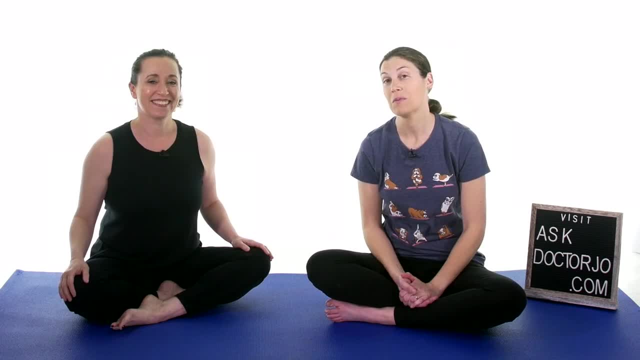 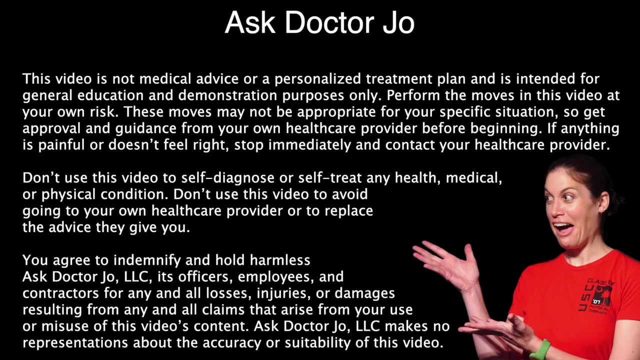 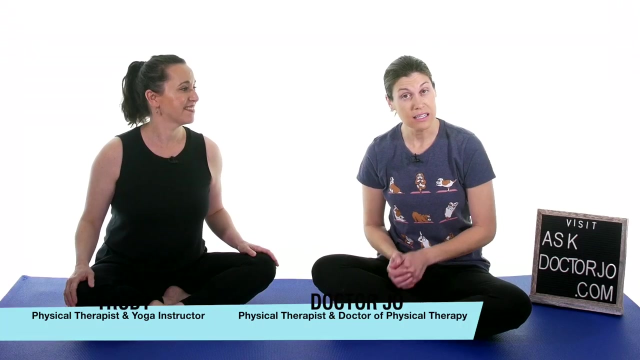 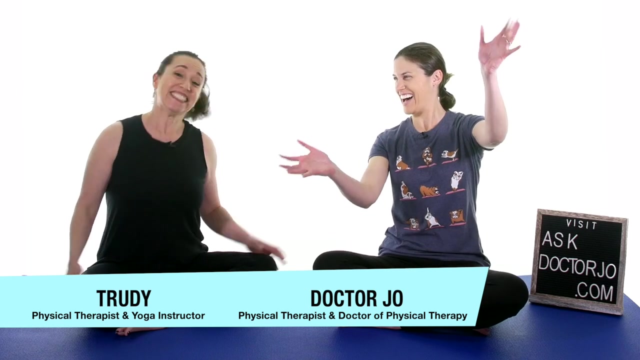 hey everybody. it's Doctor Jo and my friend Trudy, who is also one of my mentors, and today we're gonna show you therapeutic yoga for the hip, so let's get started. so Trudy is also a registered yoga instructor and she's from Canada. so, Trudy, I'm gonna have you tell a little bit about you and your. 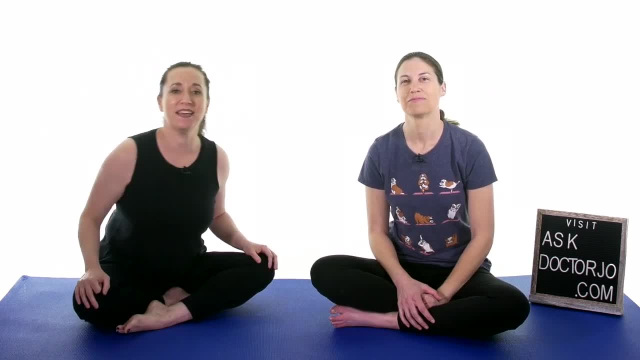 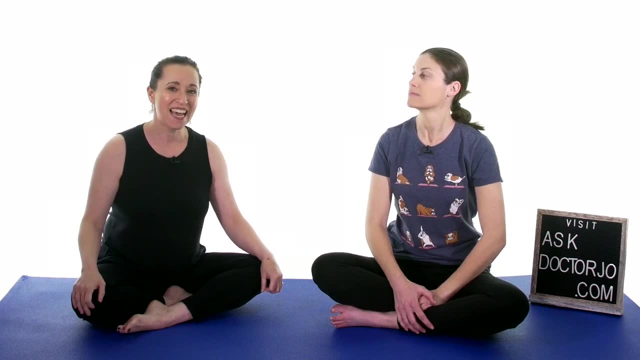 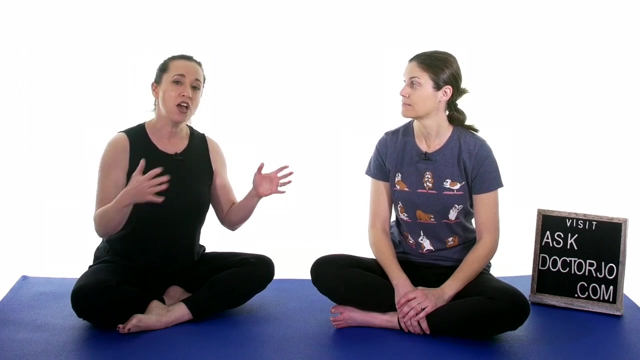 channel. all right guys. hi, I'm Trudy from Heal Wellness and Therapy. check me out on our YouTube channel, Heal Wellness and Therapy or our website, healwellnessandtherapycom. so today we're gonna be focusing on the hip joint, and the best exercises to do that are yoga-ish and physical therapy-ish for those hip. 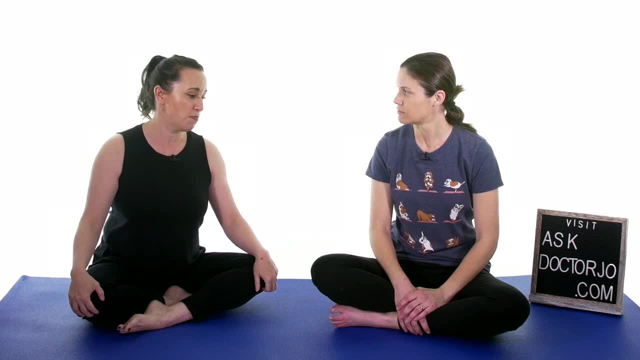 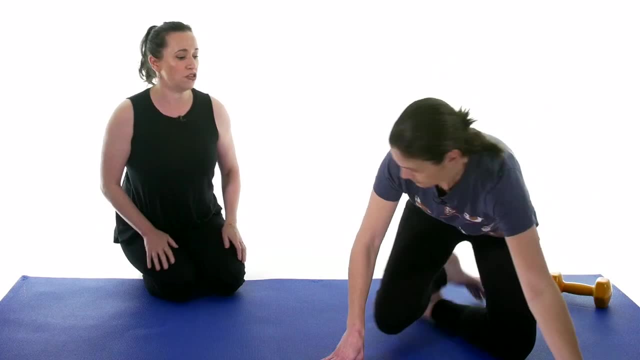 joints. so we're gonna start with a yoga pose that is called gait pose, a modification of it. so we're gonna start with a yoga pose that is called gait pose. so let's get up into a position of kneeling onto your right knee, left knee. 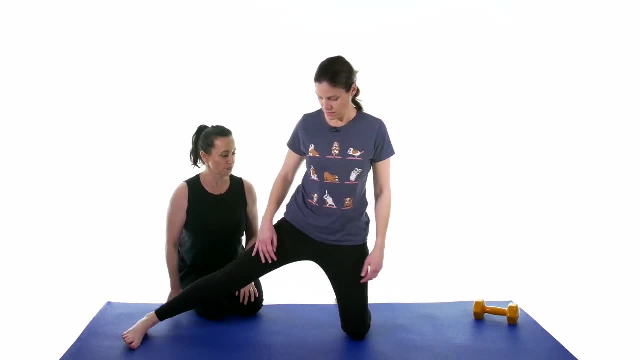 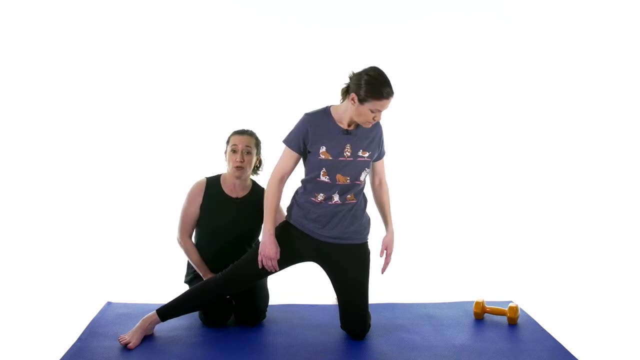 right knee, right leg, out to the side. all right now, in that position, what we want to do is make sure that the weight-bearing leg, the femur, the leg bone, is perpendicular to the floor. how are we looking there, Jo, looking good, right hand. 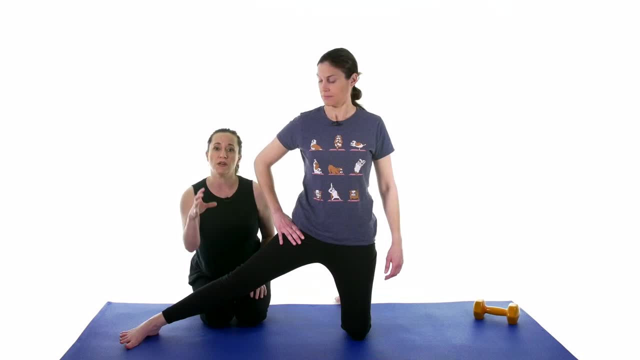 take the hand to the crease of the right hip. now here's what you're doing. whether it's hip pain, a groin strain, hip arthritis or it's just good old aging, The hip joint is a ball and socket And oftentimes what we need to do is just stretch that ball off of. 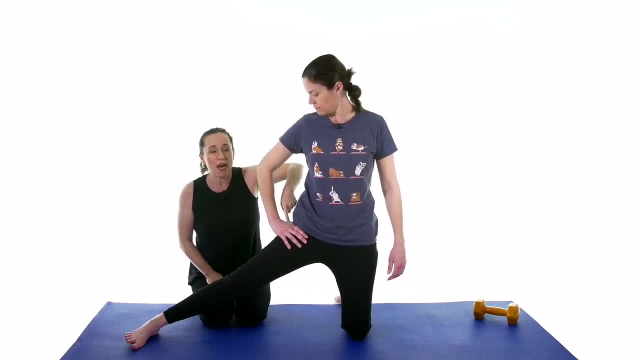 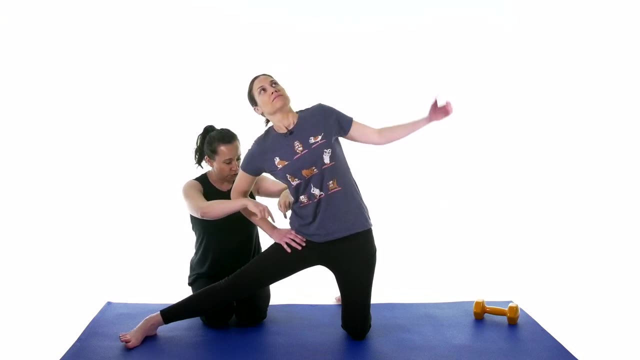 that socket And that's what we're going to do right here. So, as she weight bears that hand down into the crease of the hip, take a nice deep inhale And then, as you exhale, side bend over and pushing down into that hand- Now left arm- reach it up, Nice deep inhale And then, as you, 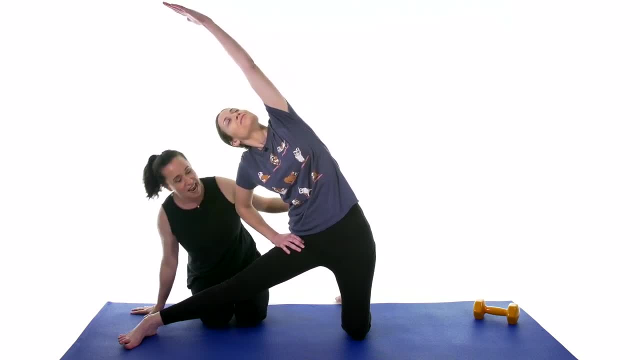 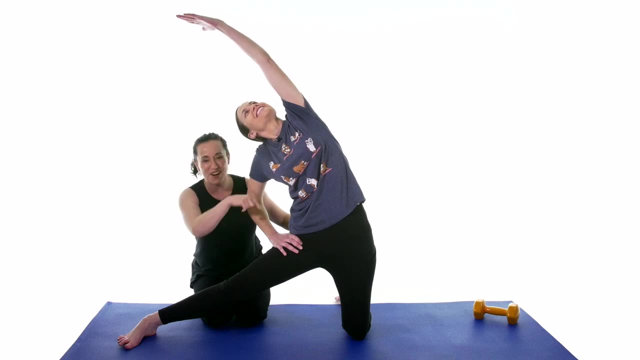 exhale side bend over even more. She's got it. Now can you? can you tuck a little bit under with that? Yes, And she just did it. She tucked her tailbone a bit to get right into that hip. 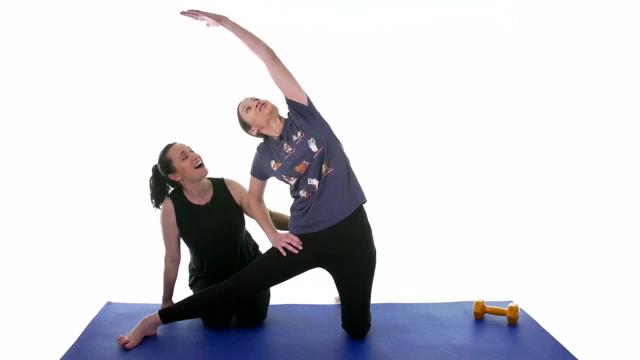 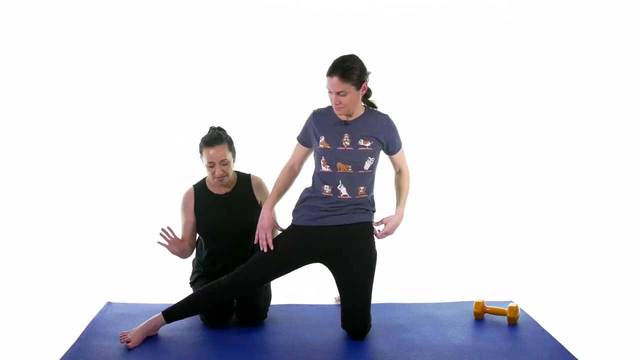 joint Holding there. Do you feel your inner thigh muscles? I do Uh-huh, Nice. deep inhale into your belly And exhaling out. One more time. Deep inhale into the belly, Exhaling out. Good left arm Inhale, Reach it high, Exhale, Relax it down And then bring that right knee in. 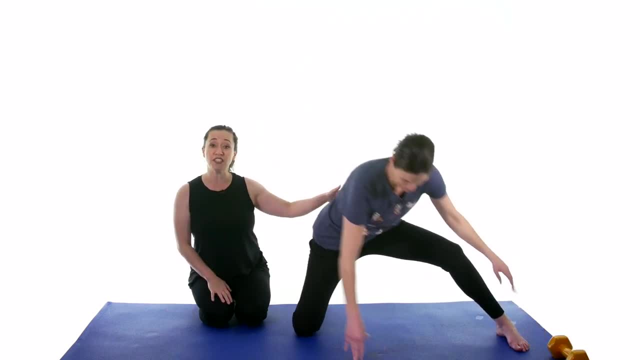 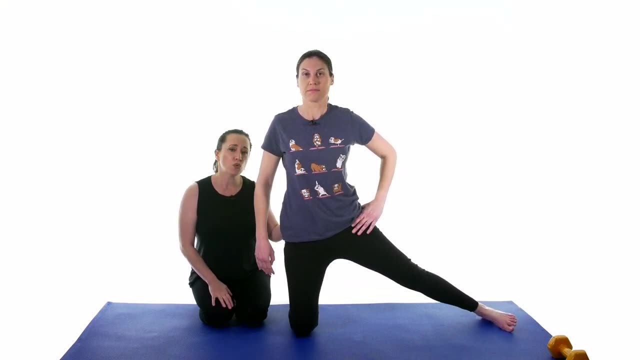 Let's do it all over on the opposite side. So left leg out to the side, Right knee vertically stacked on that hip, The foot straight behind. So real important to see that this leg is vertical, because if you're already too much in a stretch, you're not going to get this left hip as much. 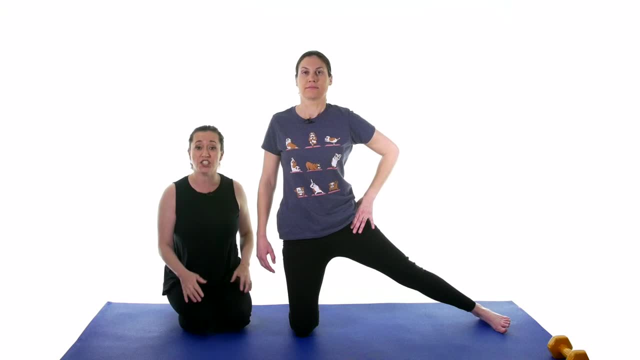 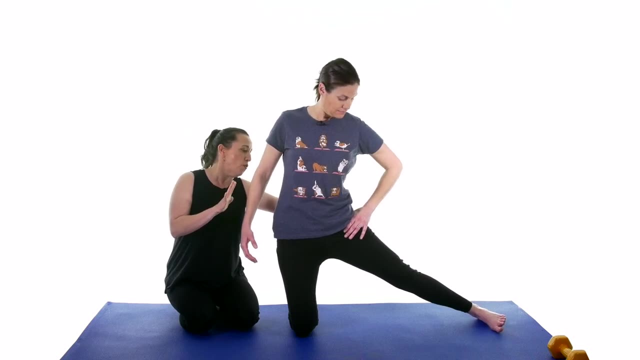 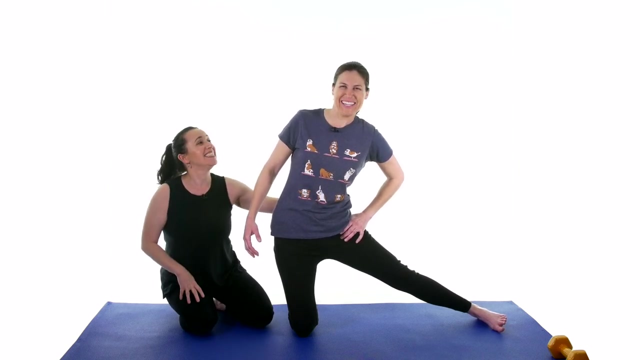 Left hand onto that hip joint while she's there, before we do anything else, Take a deep inhale And then, as she exhales, side bend up and over that hip, Push that hip down. Her hip is going nowhere. What's going on, Jo? That is my bad hip. That's a bad hip, All right. 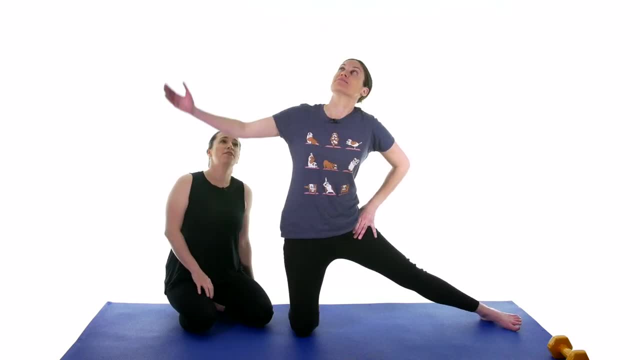 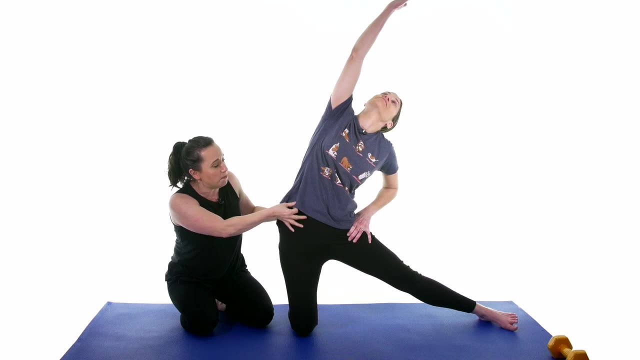 So push that hip down, what you think you can. Right arm now, without hitting knee: Inhale, Lift it up, Exhale Side, bend over. Now she is not done yet. Can you give me a pelvic tilt And 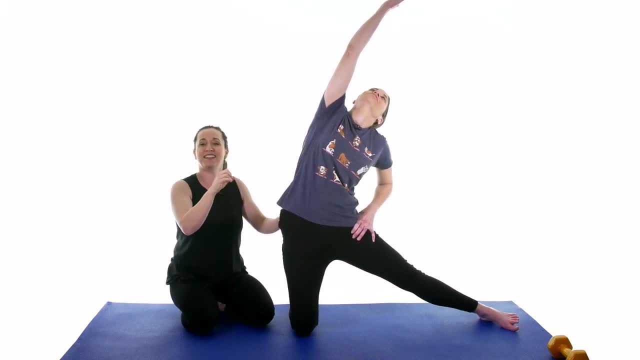 ah, there it is. Hold it there, Give me a smile and a nice deep inhale. Inhale in And exhale out. Push that hip down. Let's do that one more time. Nice deep inhale And exhaling. Then, with that right hand, inhale, Lifting it up, Exhaling it down And getting. 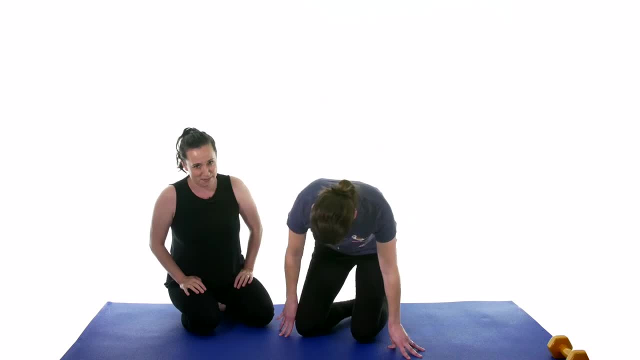 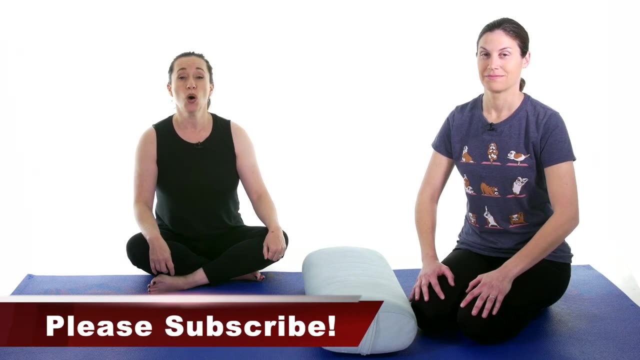 out of that left hip that she doesn't like to be in. ladies and gentlemen, All right. Now number two for the best exercises to do for these hip joints, for therapeutic yoga. We're going to tackle the psoas, muscles creating length through the front of the hip: Hip extension. 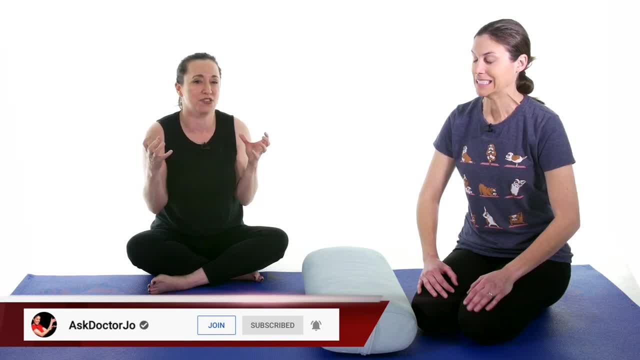 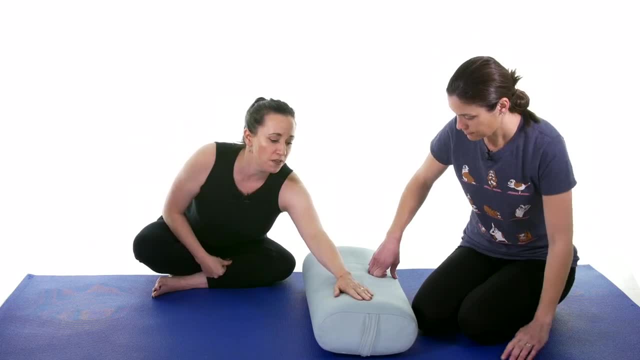 And then getting some glute facilitation or some strength through those glute muscles. So, Jo, let's get your pelvis on this bolster in an inversion. So place your hip in the front corner of that pelvis, Feet down this way And then, as you get yourself on it, 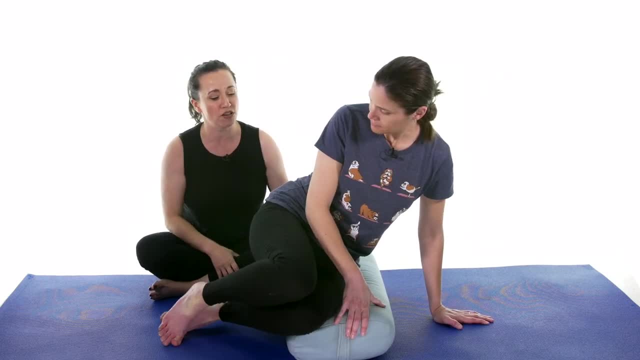 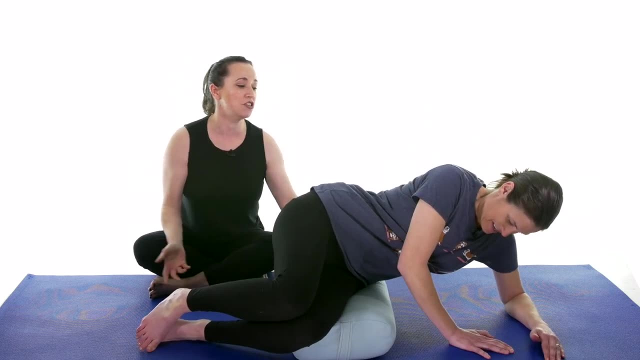 scoot yourself forward on the bolster, Because we're going to lay on your back. You've got it a little bit more. Okay, She is almost there Now. lay down on your left elbow And then, once you get there, roll yourself down onto your back And then roll yourself down. 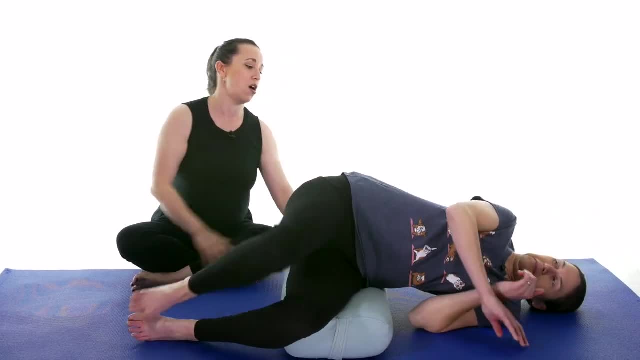 onto your right side Or lower your back, lower your body and lower your hip. So, like she can do more of that, I don't think she will find this easy, But I I like it better. now your shoulder and then over onto your back. voila, she has made it in an inversion on a yoga bolster. 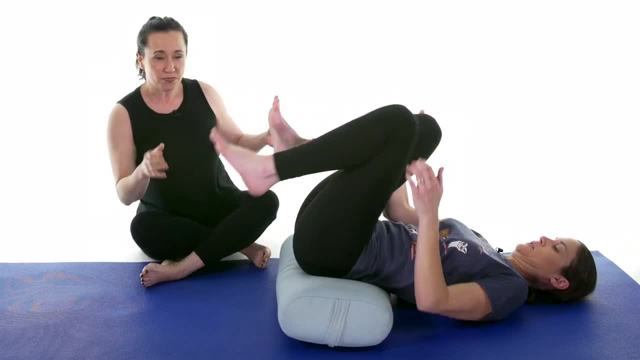 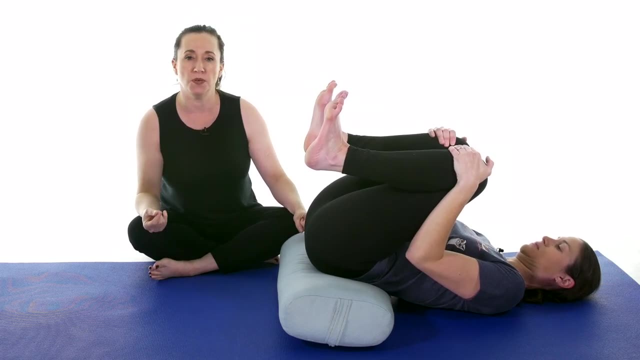 all right, so knees up to the chest to begin now. this is about the hips, so what we want to do is really create some length through the front of the hips. the number one motion people lose with walking is hip extension with a little bit of internal rotation. so that's what we want to play with with. 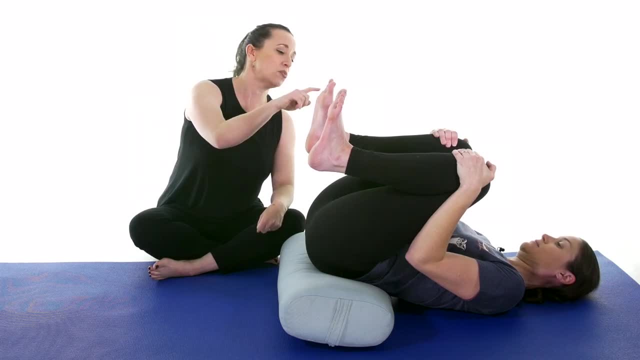 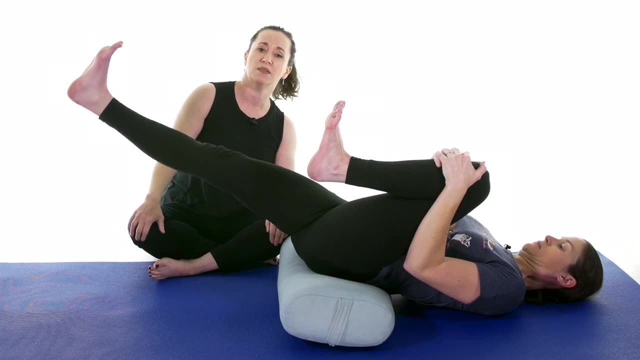 doing this particular therapeutic yoga pose. so let's start with this right leg. so keep your left knee to your chest, take your right leg, nice, deep inhale, kick that leg straight out like you're trying to knock someone out and then, as you exhale, bring that leg down to the floor. wait, is it going? 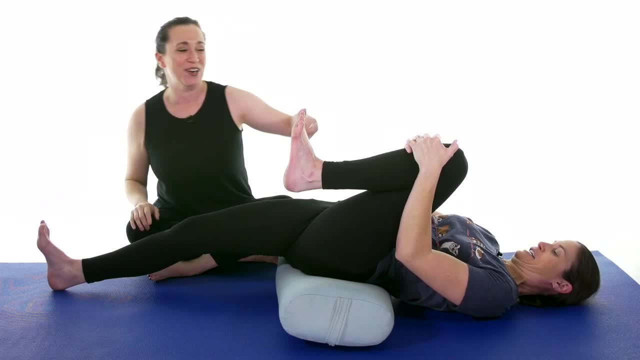 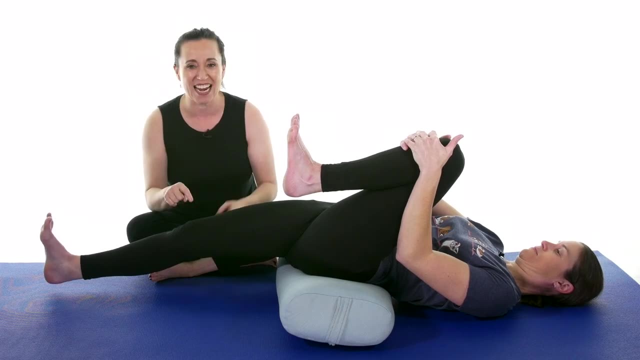 to come down to the floor. it's going to make it down to the floor. now. left knee stays into the chest, so you can see that right now we're creating this length into this right leg. her knee is bent, so i'm going to make her work really hard and then we're going to do the same thing on the other side. 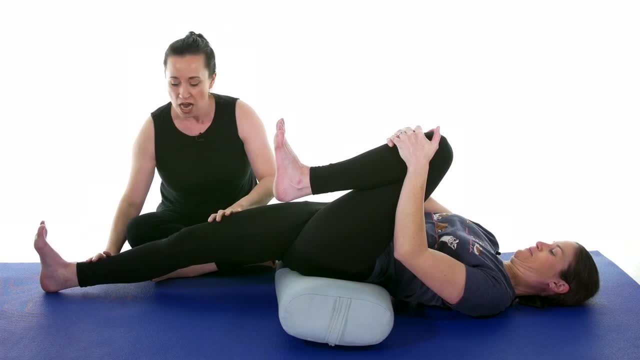 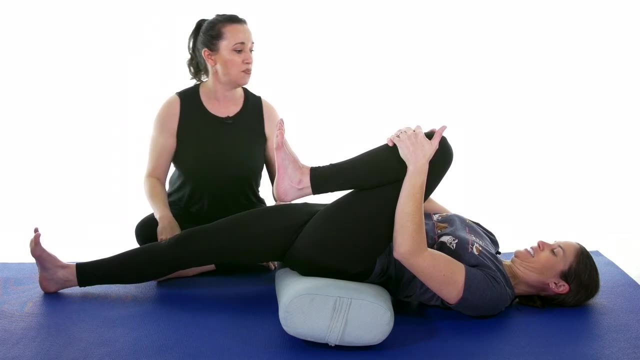 so hold the right knee straight out, strongly on your left knee and snap your right arm into the chest. okay, right knee straight out and squeeze your left knee to its내 inside really, really, really, really hard now. but before we do that, create a little bit of turning inward of your. 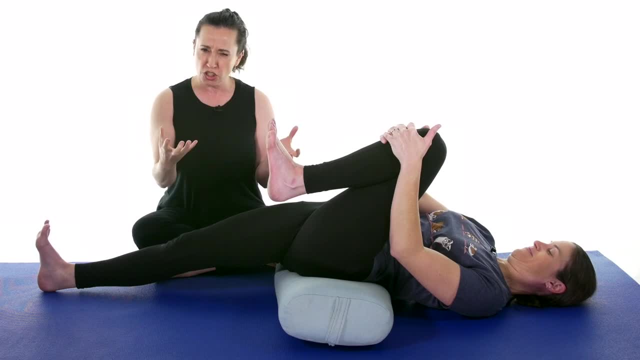 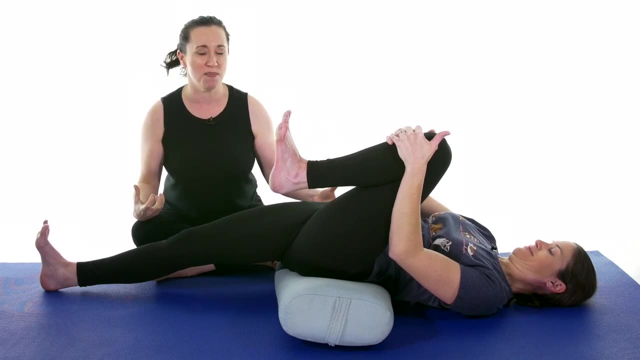 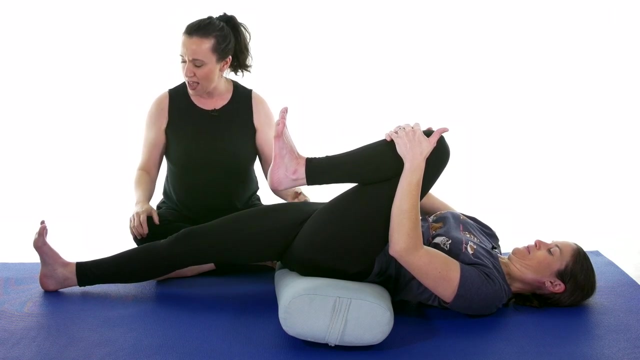 leg. so imagine your toes starting to turn inward. that's what you want. all right, are you ready, joe? all right, straighten that knee, kick that heel down and push real hard. feel your glutes engage holding that right there. give me a nice deep inhale, glutes, deep inhale and exhale. let's relax. bring the right knee back up to. 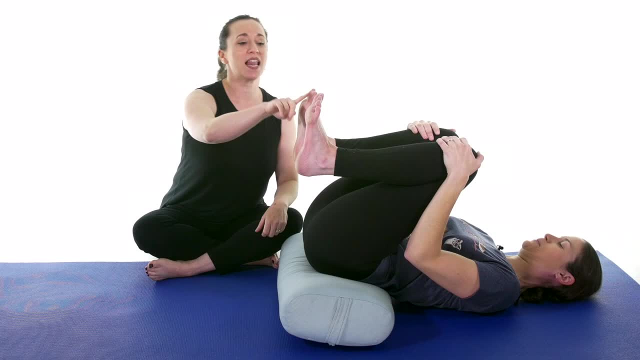 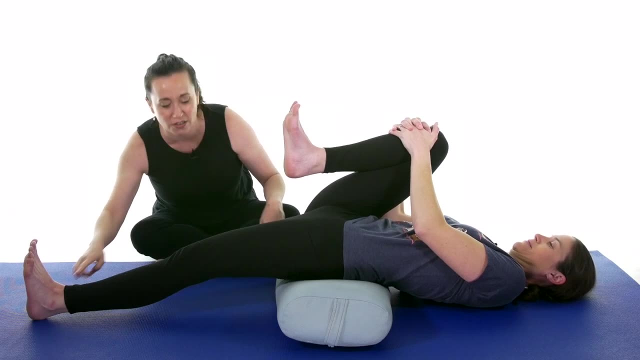 the chest. let's do it on the left, so left leg, kick it out on the inhale. on the exhale it drops down to the floor, heel to the floor, knee straight, right knee to the chest. she's faking it a little bit because this left hip is tight. 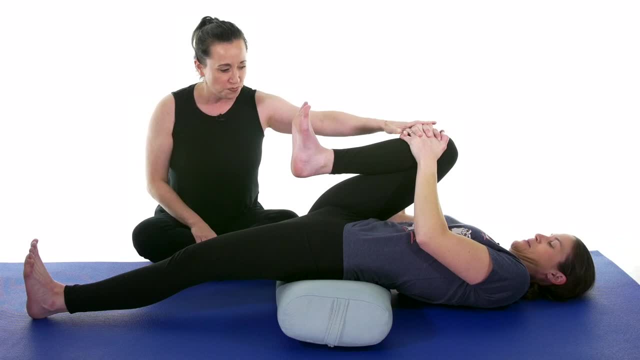 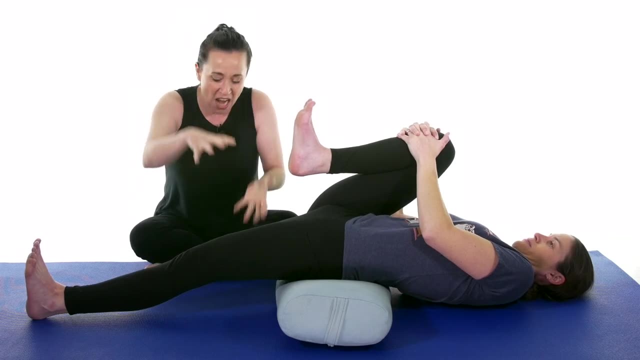 but I'm just gonna let her go with it. alright, are you ready, Jo? yep, keep that knee to your chest, keep that heel on the floor, keep that knee straight and take a deep inhale here. exhale, tighten the knee, push the leg down into the 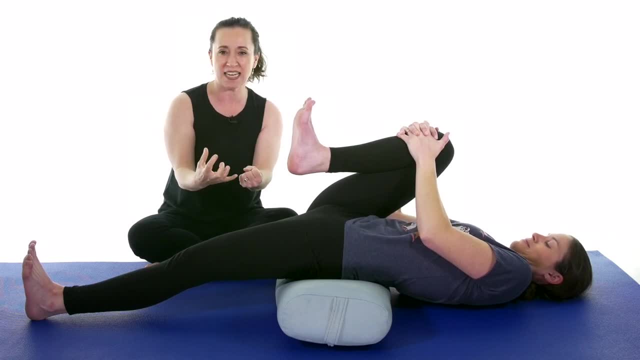 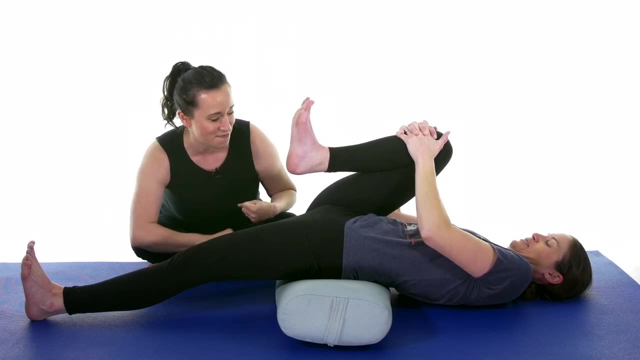 floor. feel those glutes engage, holding it there for me. nice, deep inhale into the belly, that's it exhaling. she's smiling, but I don't know if she's feeling like smiling. one more breath, deep inhale in and exhaling out, you've got it. 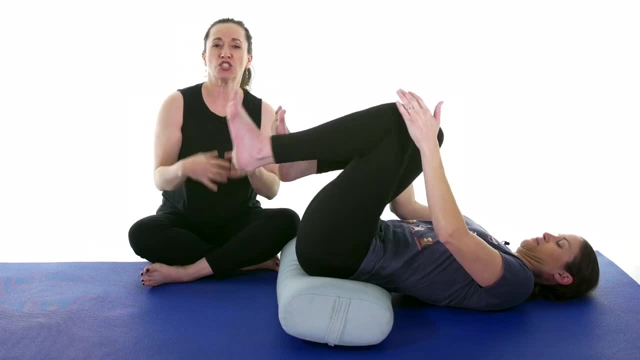 beautiful. bring that left knee back up into the chest, so doing that for multiple breaths. not only are you looking at your chest, you're looking at your body. you're looking at your body. you're lengthening the front of the hip, but you're strengthening the back of the hip. 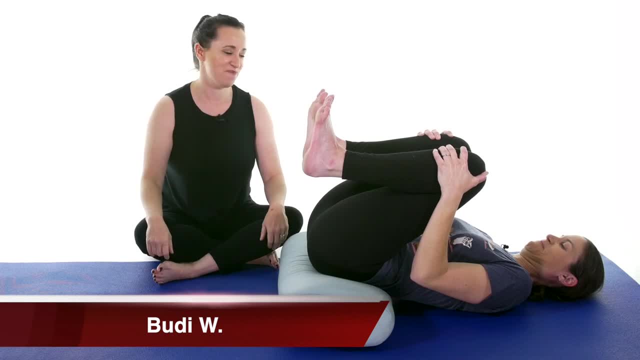 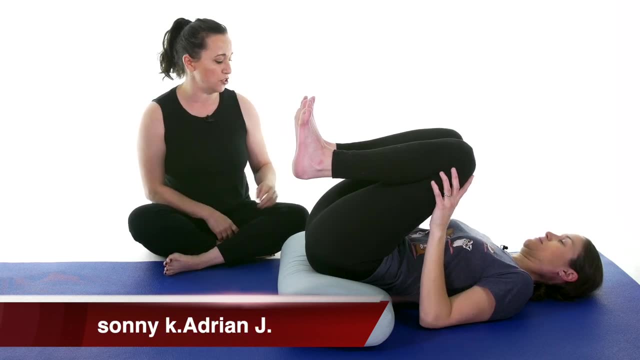 and the glutes, kind of a twofer, if you want to think of it that way. all right, last exercise for these hips. so we're gonna get ourselves off the bolster. so grab the sides of your bolster and just kind of push it and I'll take it out of. 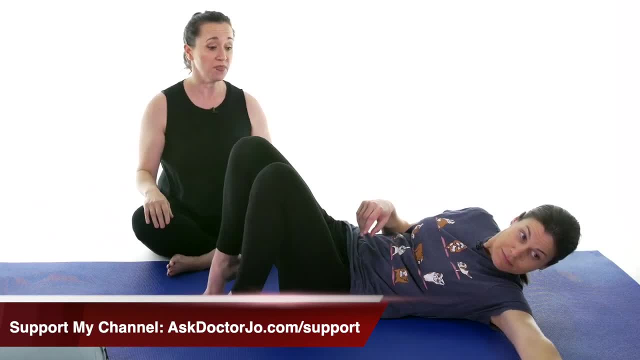 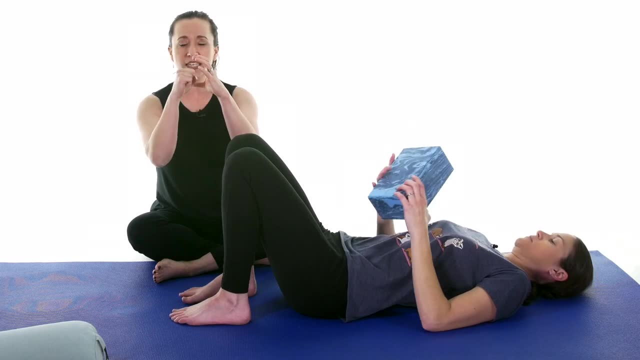 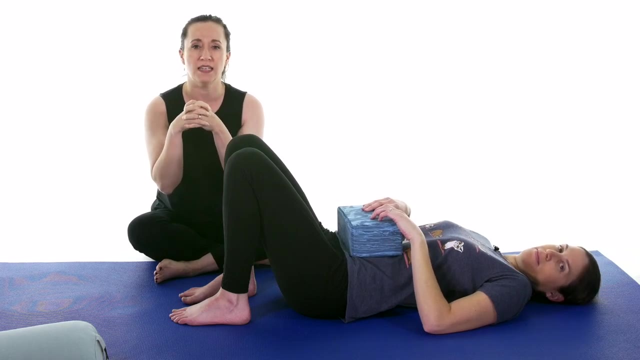 your way and then grab you a yoga block. voila, we have a yoga block, now the hip capsule, so that ball and socket has long length, lots of material keeping it nice and tense. so what we're gonna do next is a hip. 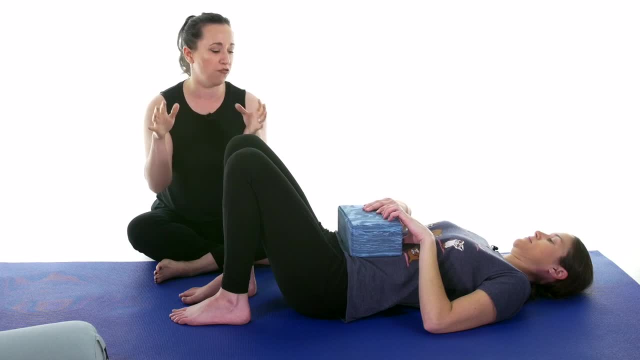 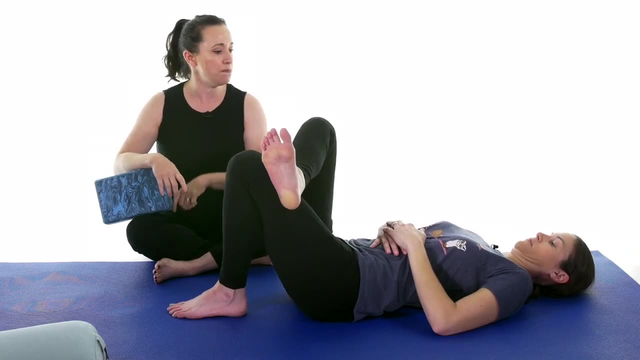 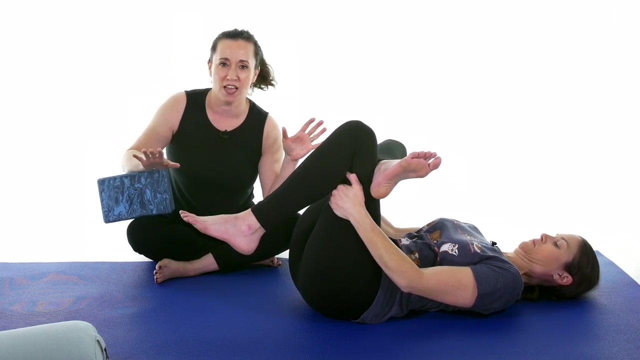 capsule stretch. oftentimes, in a fitness world, we do figure four stretches. so let me show you what a figure four stretch is. go for it, Joe. crossing that ankle over that knee, pulling that leg up and there you go. but, guys, most of us doing this we're so out of our hip and 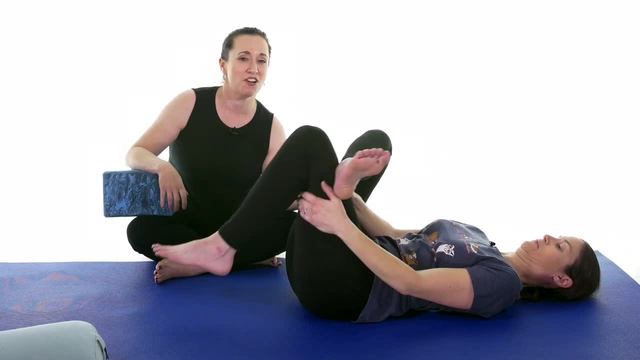 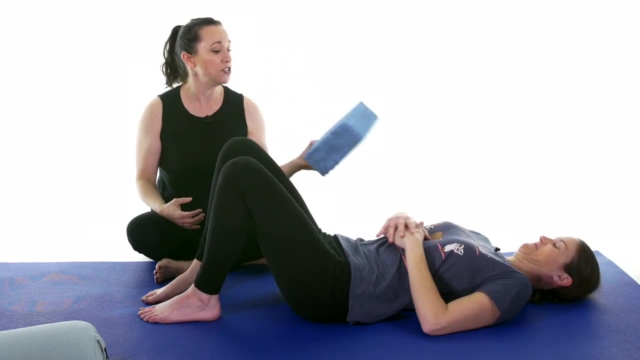 into our pelvis and our back. so let me show you the therapeutic yoga way to get these hip capsules nice and lengthened and to need a yoga block. so take your yoga block, place it in your right hand, take your left hand and sit on it. so 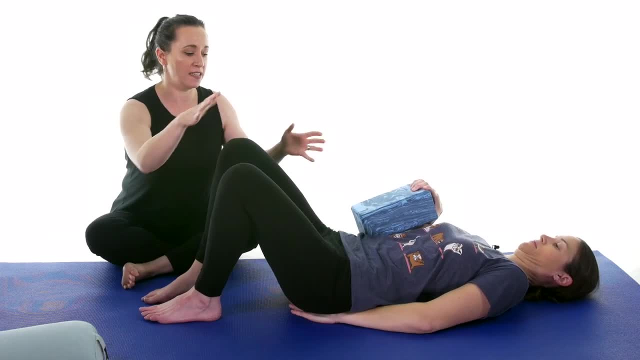 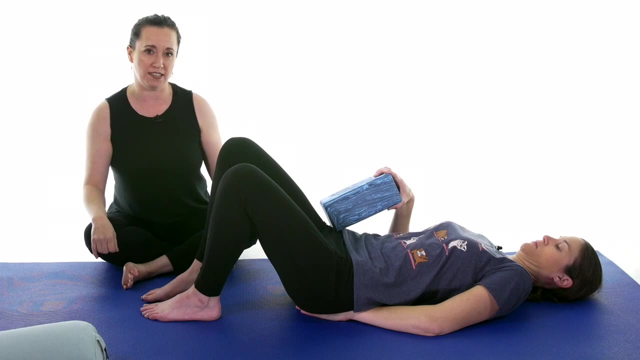 place your left hand underneath your bottom. now what that does is it promotes the pelvis and staying neutral. so she's not gonna let the pelvis rotate when she crosses this leg and the ankle up and over that knee. so go ahead and cross it. 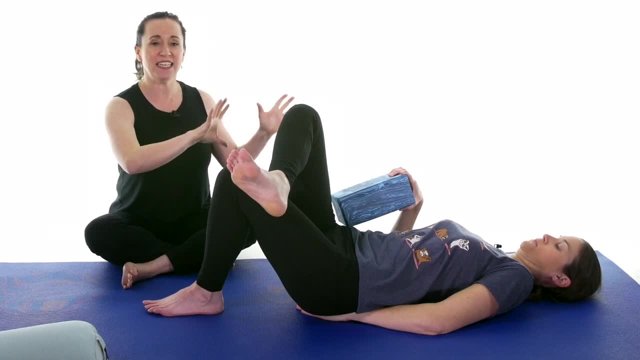 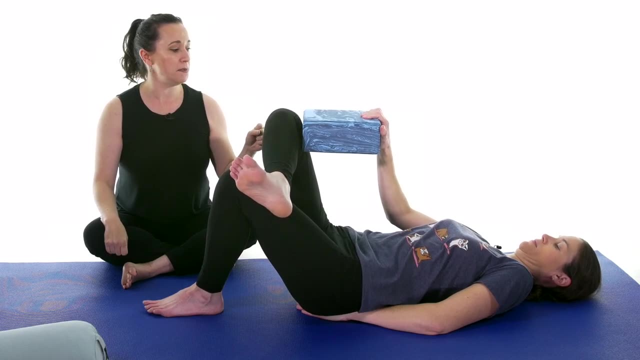 now sit into that left hand. you've got it. see how everything kind of moves to the left. that's what we want. block onto the knee, holding yourself right here. now take a nice deep inhale and then, as you exhale, gently push the knee away until you feel. 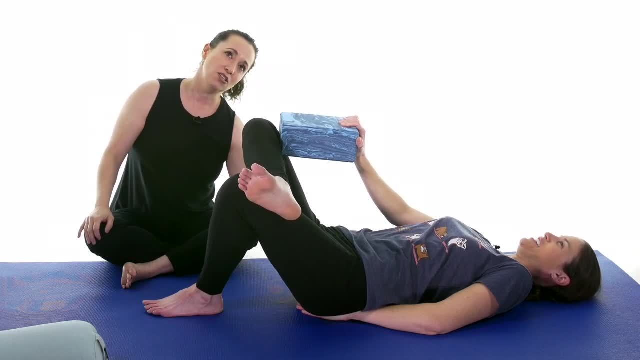 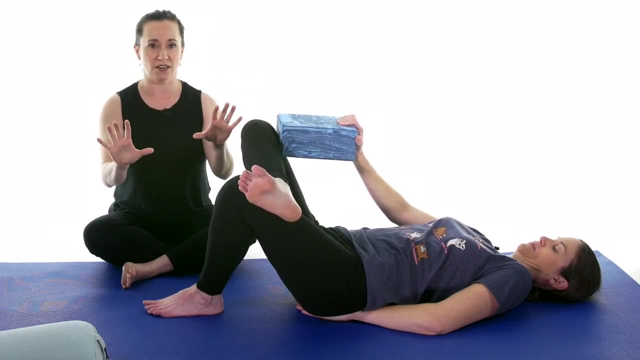 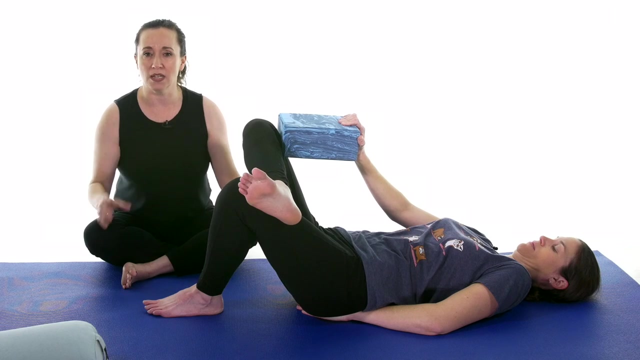 it in the outside of the hip. Joe, feel it in the outside of the hip. we're doing it right. so sit into the left hand, push into the right knee, hold it all right there, take a deep inhale into the belly and exhaling out real slow exhale relaxes that hip. 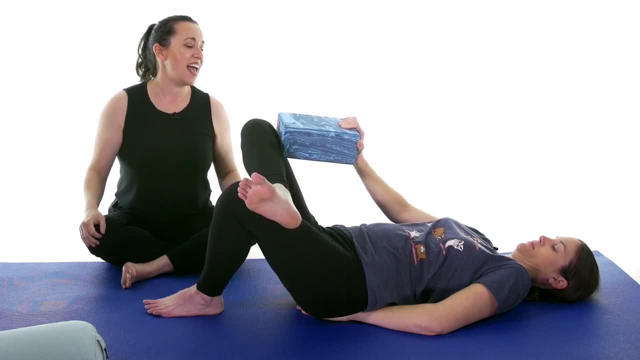 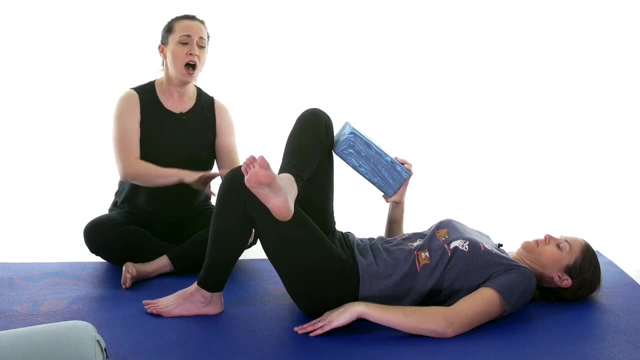 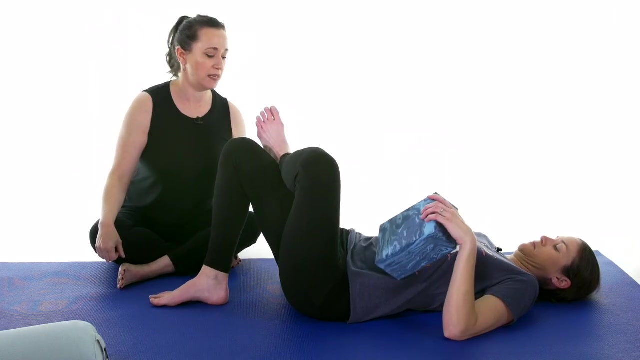 capsule even more nice: deep inhale in and exhaling out, beautiful, releasing the block, taking the left hand from underneath you, uncrossing that leg. let's try it on the opposite side. so left ankle over right knee as left knee bends. 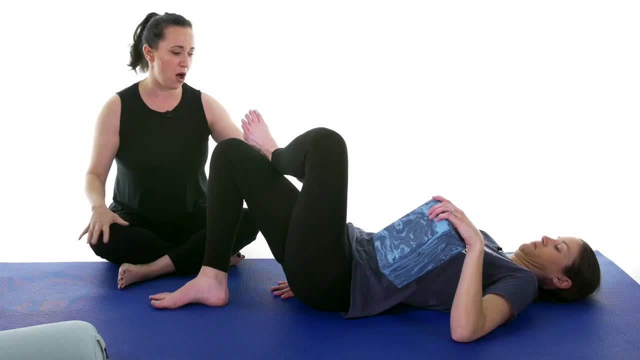 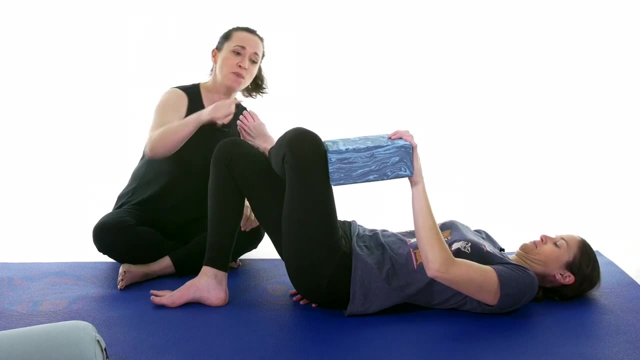 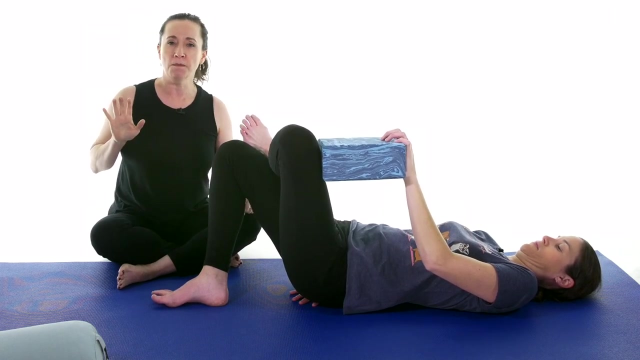 right hand underneath the bottom and sit on that bottom. stop that pelvis and lumbar spine from rotating. then take that yoga block or whatever you got that looks like a yoga block at home, place it against that leg, left knee now sitting into that right hand. nice, deep inhale here and then as 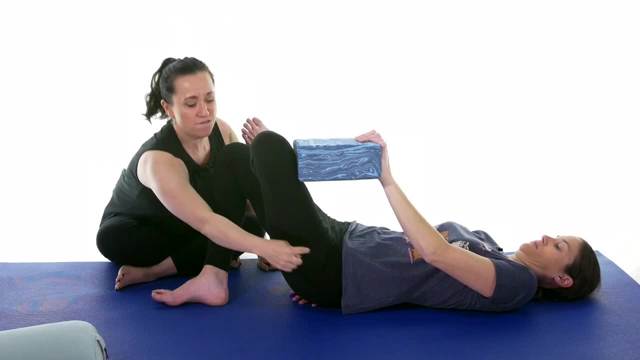 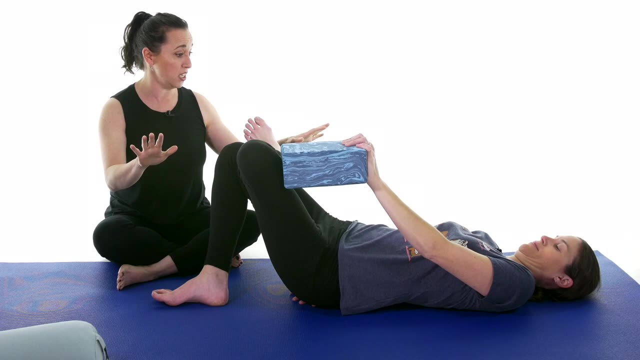 you exhale, start to push that knee away, feeling that stretch right out here, getting that hip capsule exactly where we need it, how we feeling good, got it sitting into the right hand. let's do two deep diaphragmatic breaths here, deep. 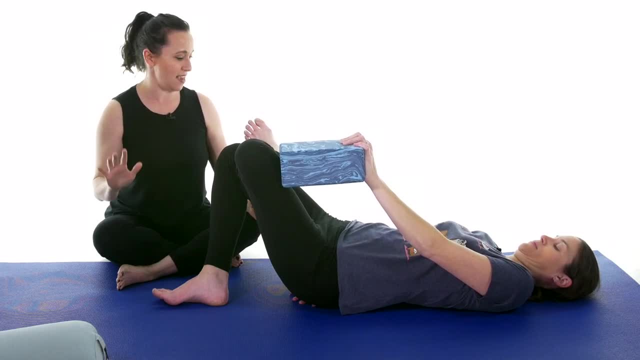 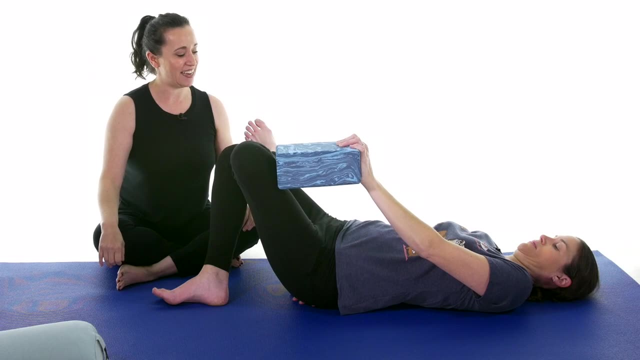 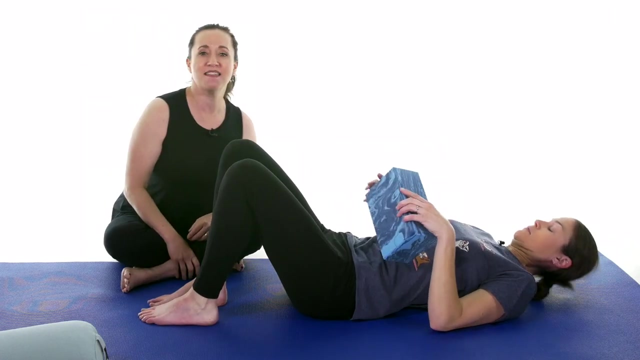 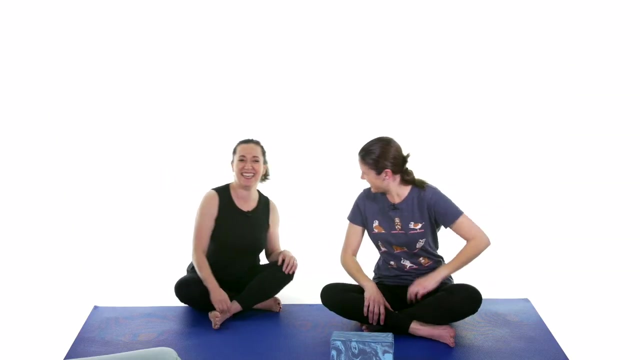 inhale in, slow, relaxing, exhale out. you've got it one more time. nice, deep inhale in and slowly exhaling out. beautiful, releasing the block, releasing the hand, uncrossing the legs and the most perfect hips are here with us now. so there you. 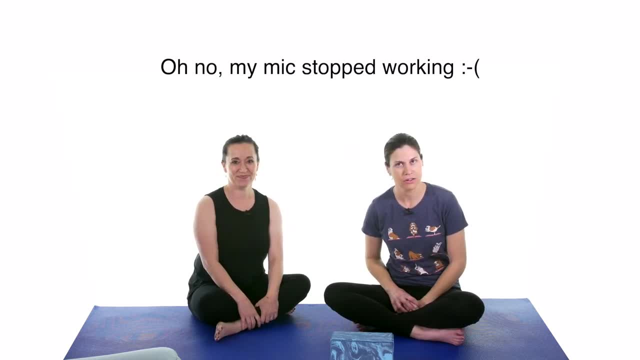 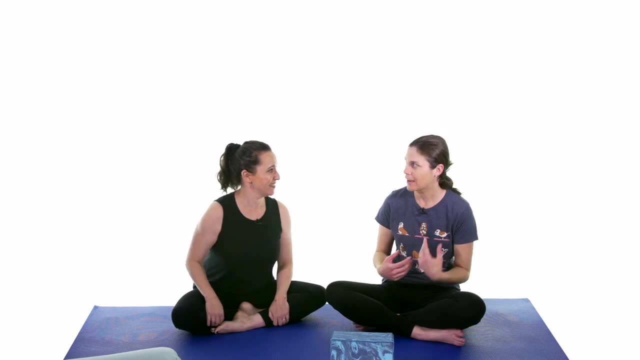 have it. if you'd like to help support my channel, make sure and click on the link over there. and don't forget to subscribe by clicking down there. and remember, be safe, have fun and I hope you feel better soon. and hey guys, it's a therapeutic yoga class, so let's end the yoga way hands to heart. 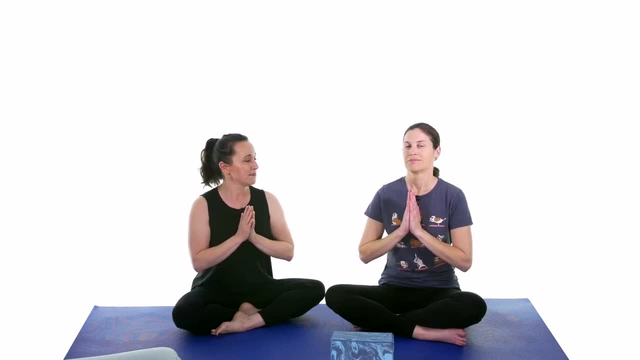 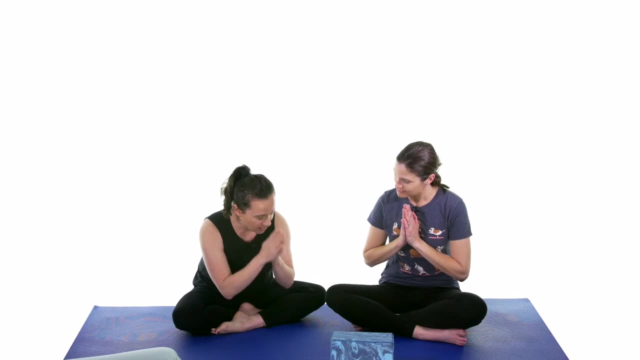 smiles on our faces. nice deep inhale in and exhaling out. namaste, the highest in me salutes the highest in you.